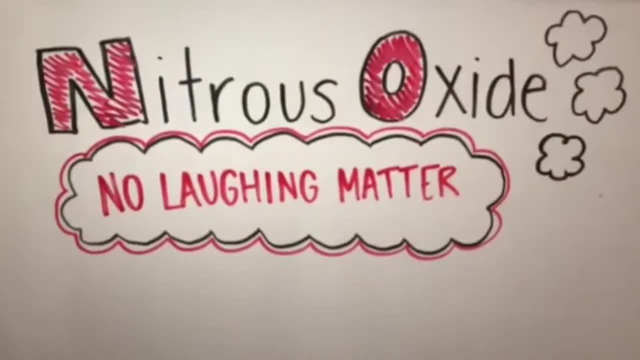 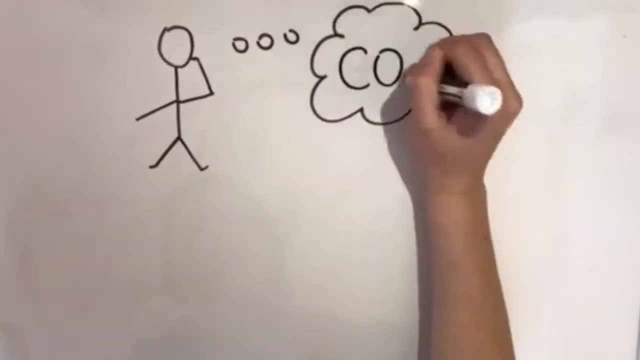 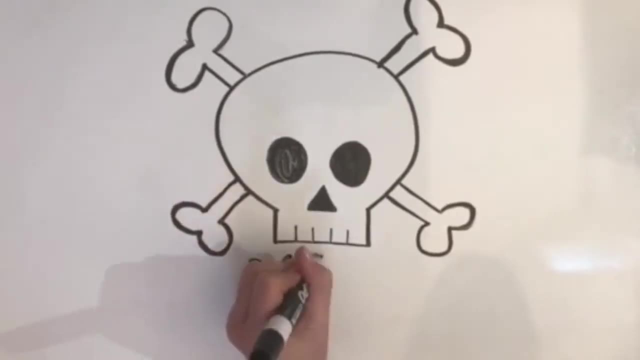 When you think of greenhouse gases, most people think of carbon dioxide. This makes sense, as carbon dioxide accounts for 80% of human-emitted greenhouse gases. But did you know that there are more dangerous greenhouse gases, such as nitrous oxide, out there? This unawareness, 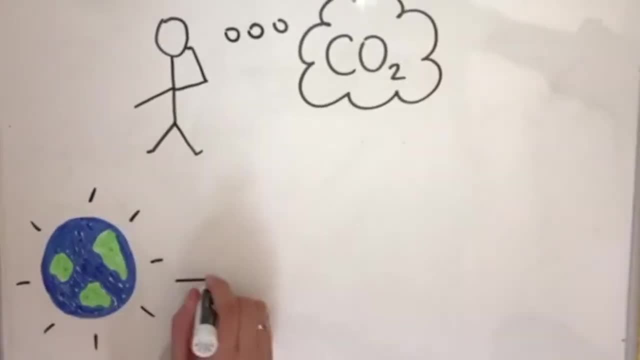 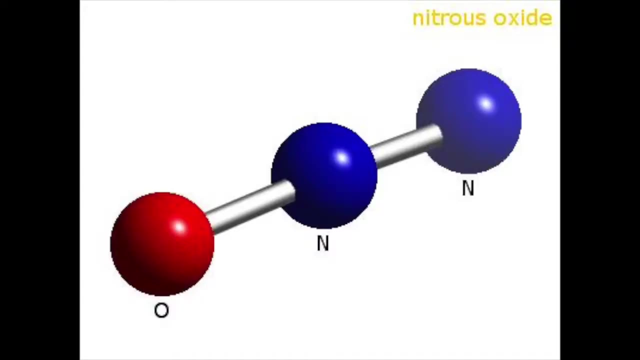 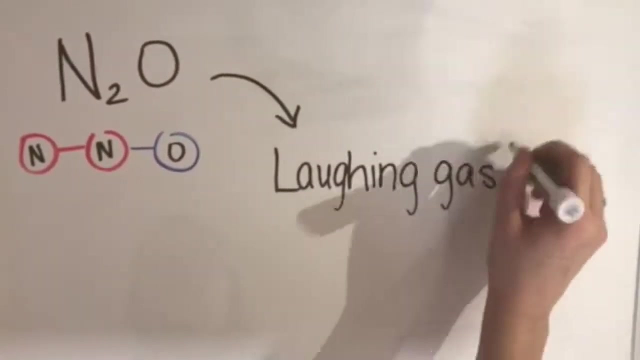 of other greenhouse gases could lead to the downfall of our environment, our economy and our health. Nitrous oxide is a small chemical compound comprised of only two nitrogen atoms on one oxygen atom. You might know this as laughing gas. It's hard to believe that this. 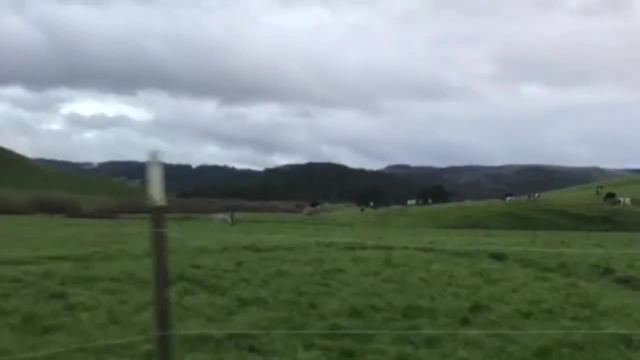 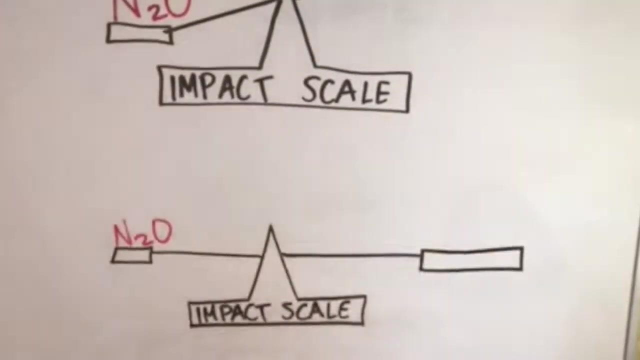 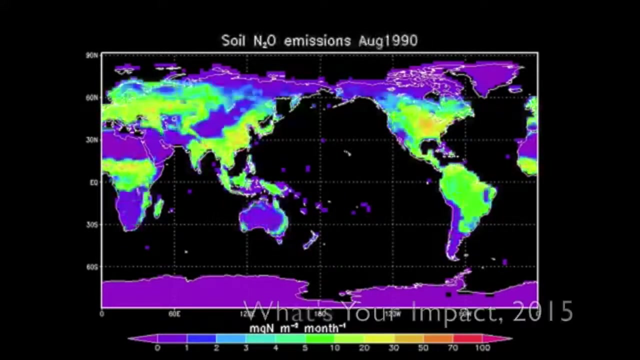 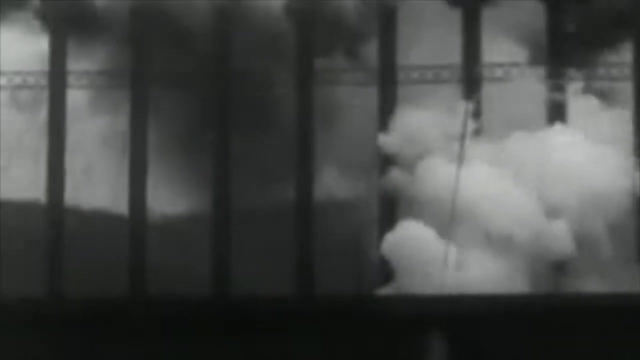 small molecule is really an extremely potent greenhouse gas. In fact, one nitrous oxide molecule has the same impact as 310 carbon dioxide molecules. Current nitrous oxide levels are the highest they've ever been during the last 800,000 years. The atmospheric concentration of nitrous oxide began to increase during the industrial 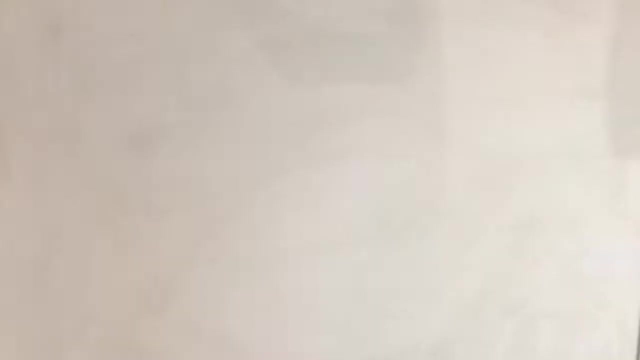 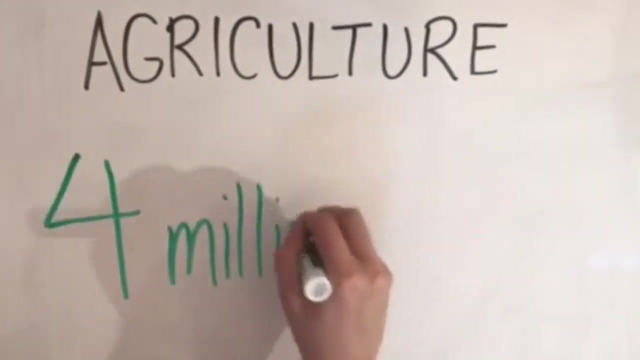 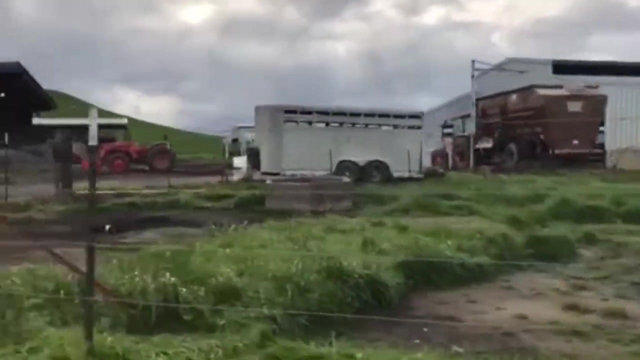 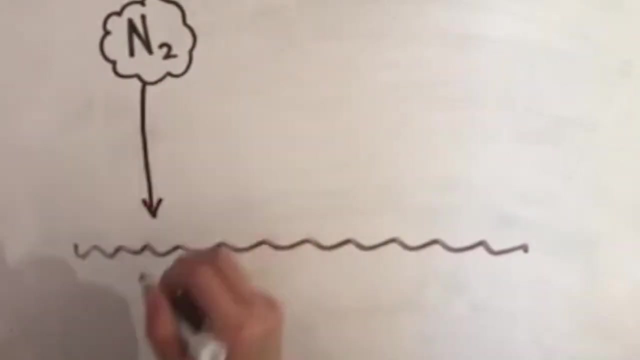 revolution due to human activities. You may not realize that agriculture is the number one human activity that emits nitrous oxide, releasing almost 4 million tons per year globally. That's 67% of all human nitrous oxide emissions. Let's take a look at the chemistry behind nitrous oxide in the nitrogen cycle: Nitrogen. 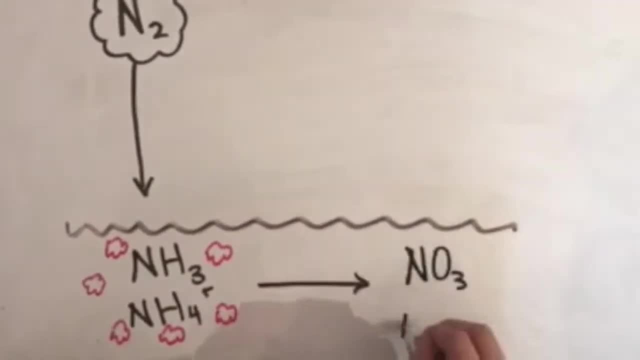 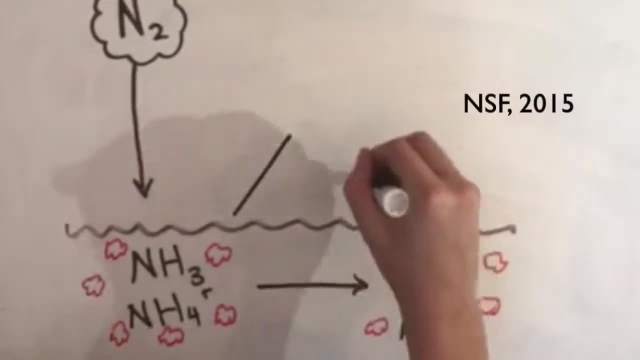 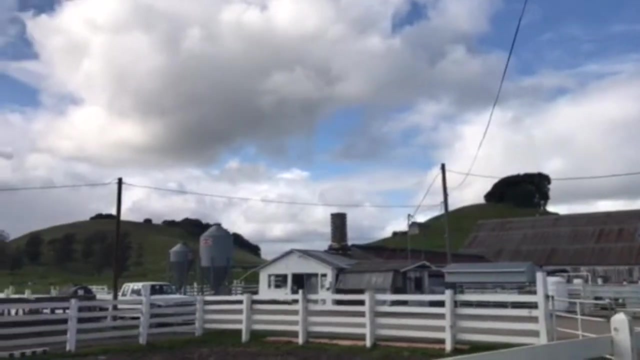 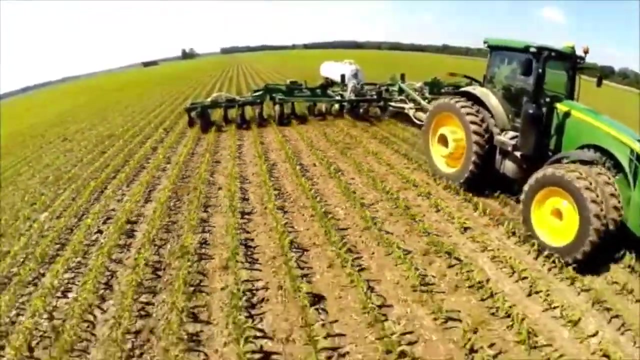 gas in the air is converted into ammonia and ammonium and then nitrate and nitrite ions by bacteria in the soil. During this process, nitrous oxide is released as a by-product into the atmosphere. Agricultural practices amplify the nitrous oxide emissions greatly. Synthetic nitrogen-based fertilizers that are commonly used on crops 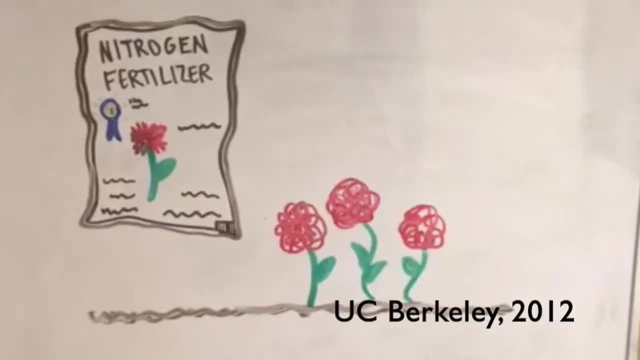 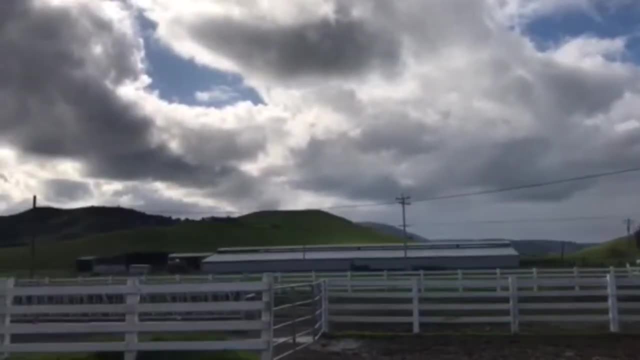 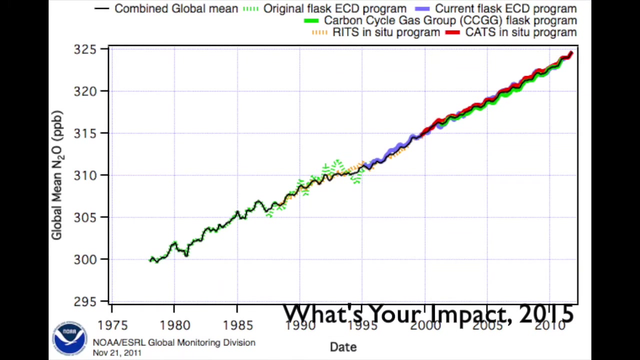 increase the nitrogen in the soil and therefore increase nitrous oxide emissions. In fact, there is a direct correlation between the increased use of nitrogen fertilizers used by industrial agriculture and the increase in nitrous oxide emissions. One of the many solutions to nitrous oxide emissions is the use of nitrogen-based fertilizers. Nitrogen-based